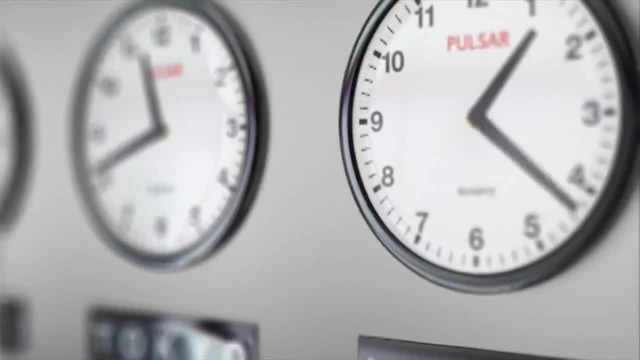 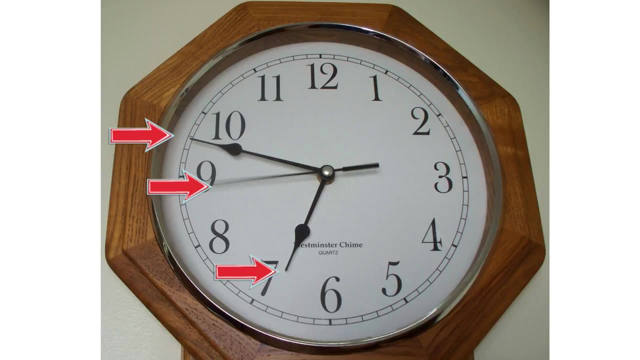 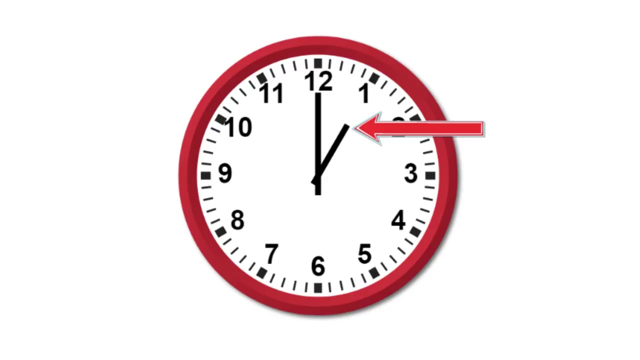 Welcome to MooMooMath and Science. In this video let's learn how to tell time on an analog clock, And on this video we are going to focus on a clock with three hands. The small hand is for the hour. It points to the hour and there are 24 hours in a day. You always start. 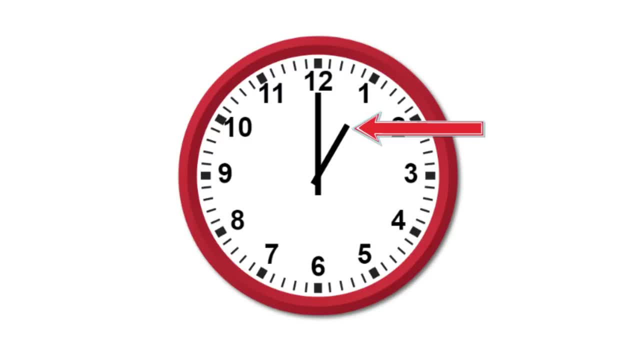 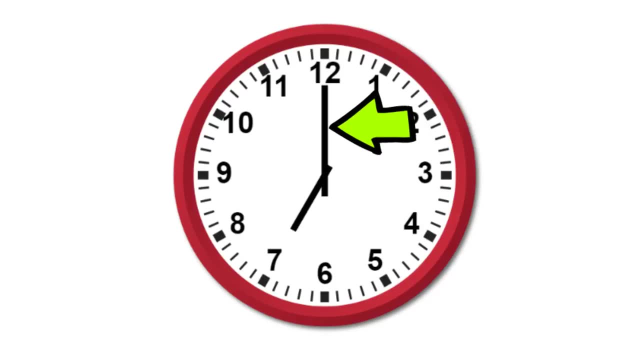 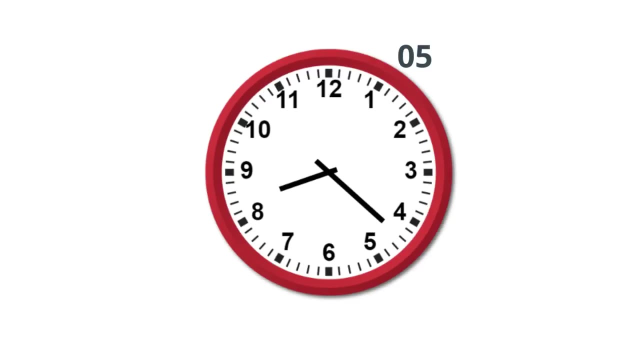 with the shortest hand or the hour hand. This is one o'clock, three o'clock, seven o'clock. The large hand tells you the minutes. There are 60 minutes in an hour. For each number it is equal to 5.. So you have 5, 10,, 15,, 20,, 25,, 30,, 35,, 40,, 45,, 50,, 55 and the last number. 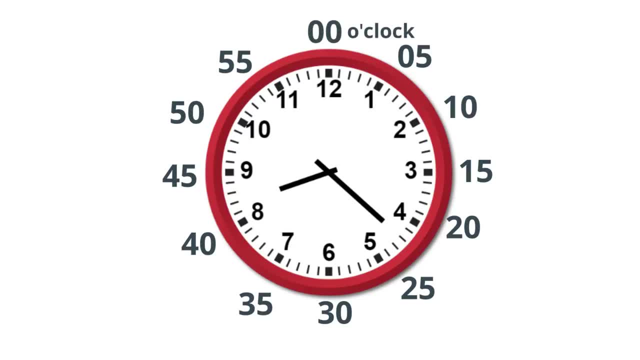 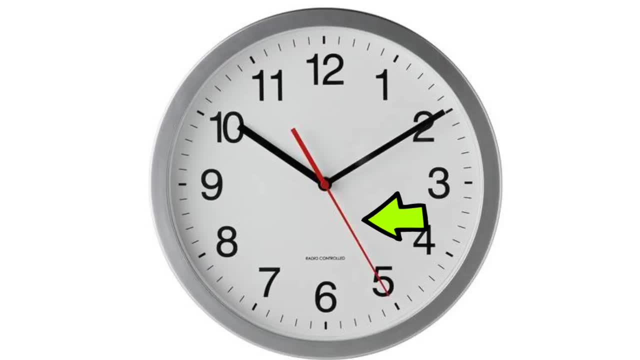 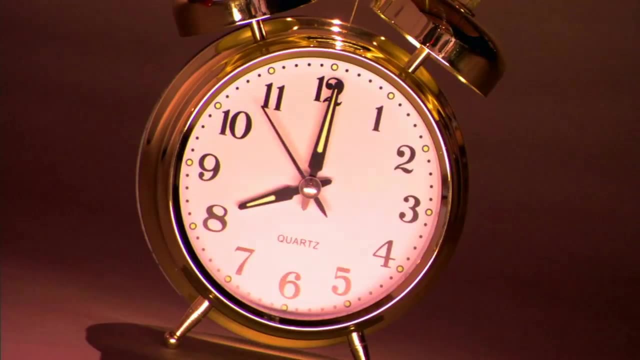 is two zeros, not 60, and you call it o'clock. The third hand tells you the seconds. There are 60 seconds in an hour. The second hand moves more quickly than the hour and minute hand and sometimes it may be a different color, like red, or it may be thinner than the hour and minute hand Use. 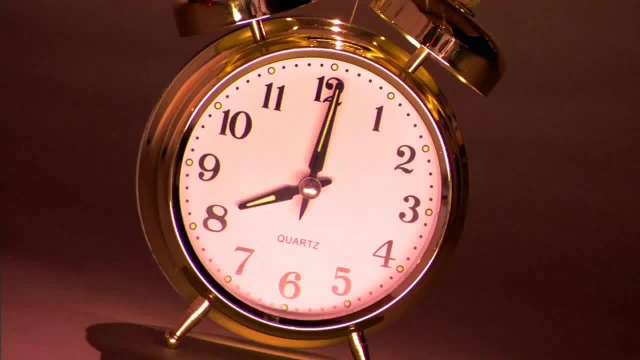 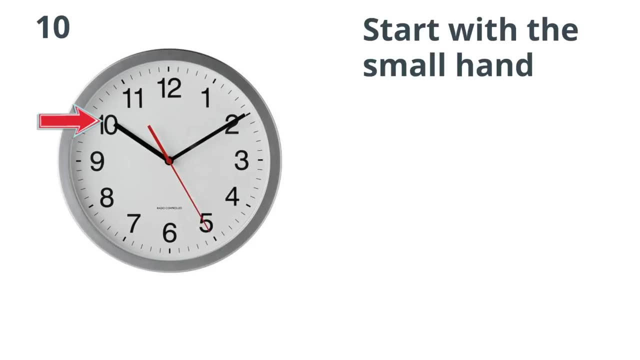 these five steps in order to make reading time easy on a clock. Step 1. Start at the small hand, Look where the short hand is pointing and write this down. Step 2. Draw two dots. Step 3. Read the large hand. 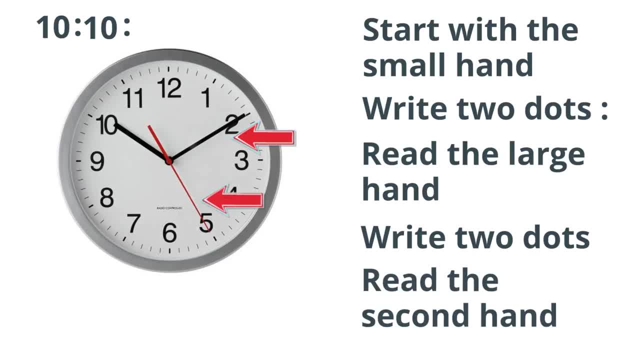 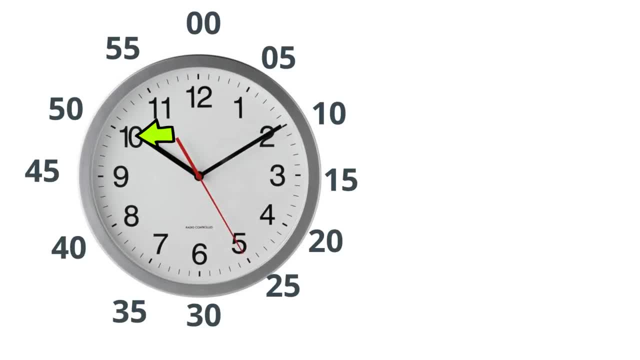 Step 4. Draw the short hand. Step 5. Read the skinny or the second hand. So let's practice This first one. the small hand is on the 10. Let's write down two dots. The large hand is at 10 also, So let's write a 10.. Now, the second hand is on the 25. So 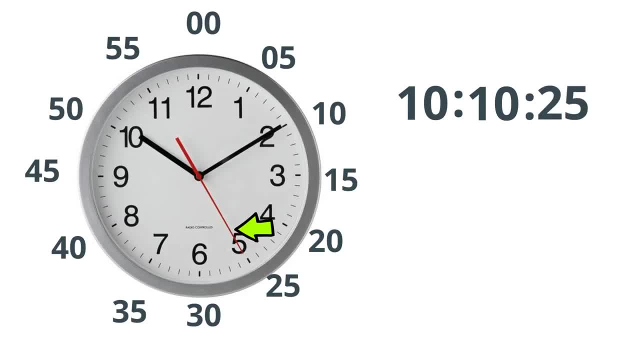 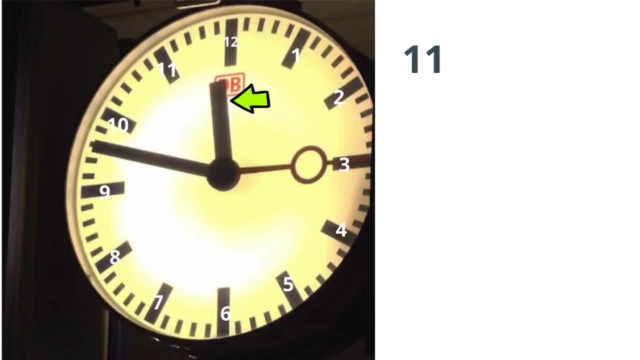 let's write 25.. So there we go. Let's go with the second one. The small hand is on the 11. So I'm going to write an 11, then two dots. The large hand is on 48. So how did I get the 48?? This is 45, then 46,, 47, 48. I'm going to write two.